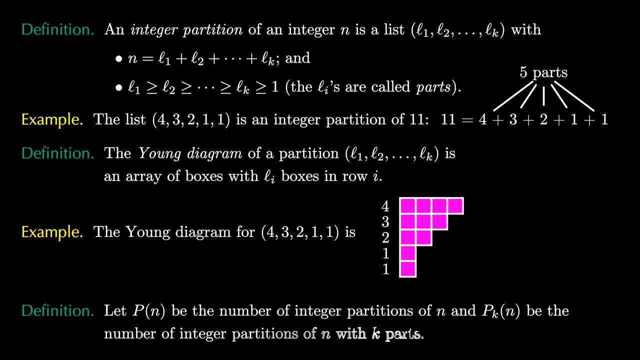 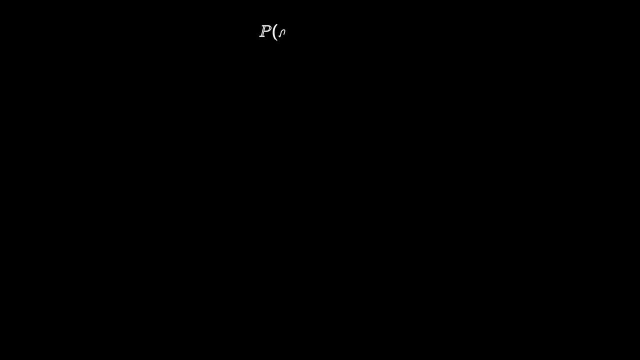 and then one. Let's let p of n be the number of integer partitions of n and p sub k of n be the number of integer partitions of n with k parts. If we're trying to compute p of n, we can list out all of the young diagrams for n, In this case. 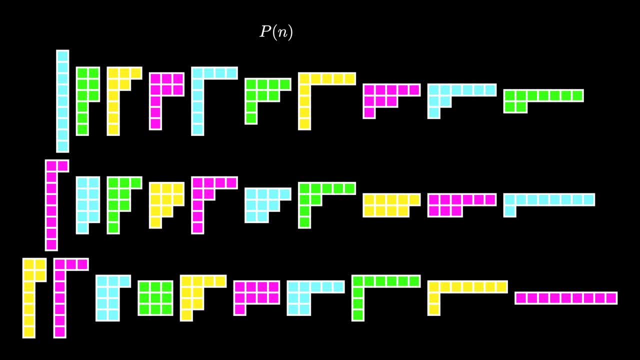 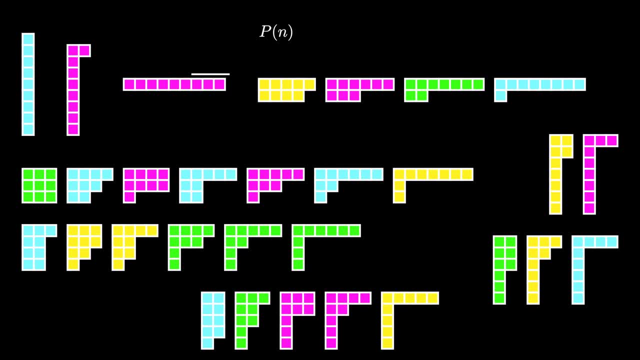 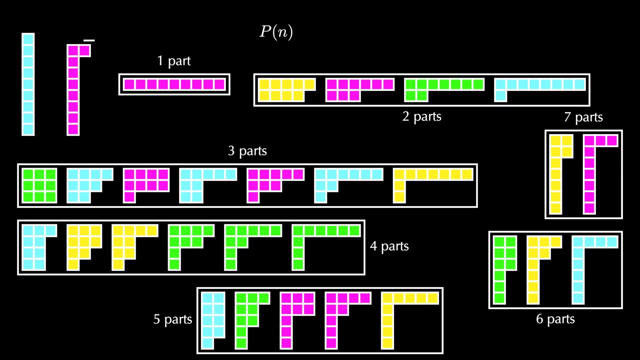 we have n is nine, and here are all the partitions. A natural way to organize the partitions is to group them together with other partitions with the same number of parts, as we've done here. The smallest number of parts a partition can have is one, and the largest number of parts it can have. 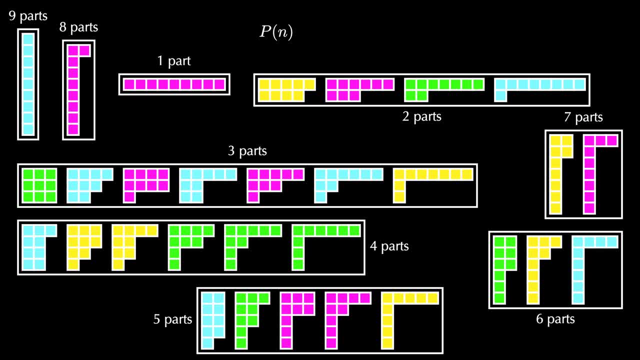 is n, where each part has size one. This visual shows us that the number of partitions of n is equal to the sum of the number of partitions of n into k parts, where k ranges from one to n. Now we can present our primary result about the number of partitions of n into k parts. 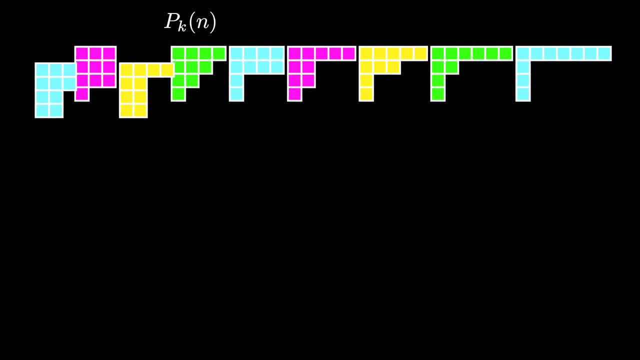 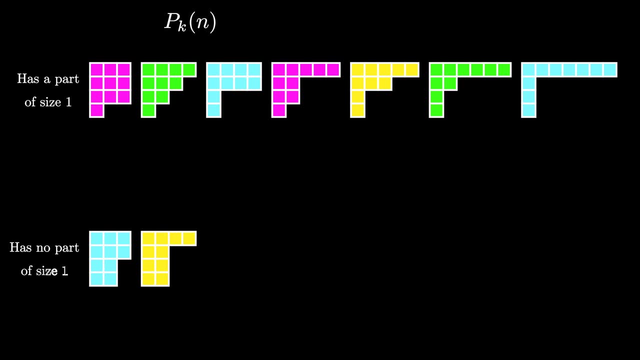 If we have all the partitions of n into k parts, we can divide these into two disjoint sets. The first set are the partitions that have a part of size one, and the second set consists of the partitions with no part of size one, The partitions that have a part of size one. 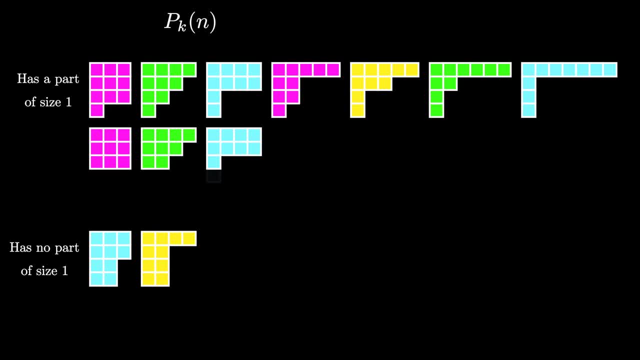 are in one-to-one correspondence with those partitions where we remove one of the parts of size one. But these partitions are just the partitions of n minus one into k minus one parts, so we can count them using p sub k minus one of n minus one For each of the partitions that have. 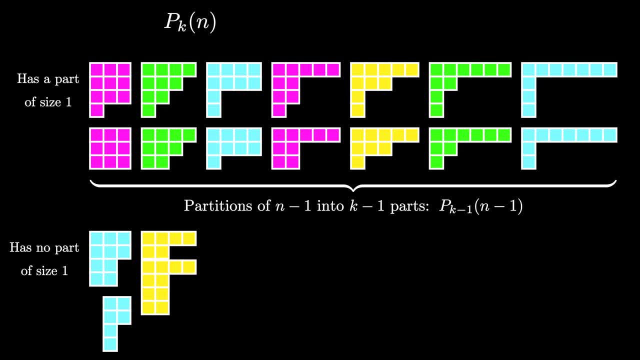 no part of size one. we can remove one from the set of partitions of n, minus one from each part, resulting in a partition of n minus k into k parts. These can be counted by p sub k of n minus k. Both of these processes are reversible and because the two sets have 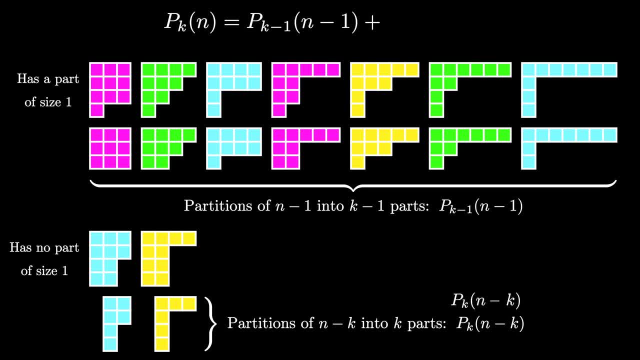 no elements in common. we see that p sub k of n is equal to p sub k minus 1 of n minus 1, plus p sub k of n minus k. This is a recursive formula for p sub k of n, the number of partitions. 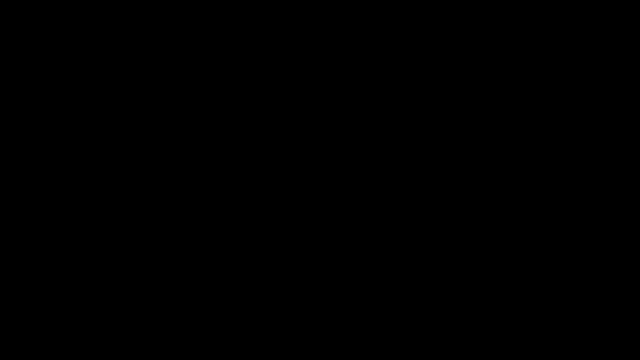 of n into k parts. We now see that we do not need to enumerate all of the partitions to know how many there are. Instead, we can use the two formulas that we just encountered to find the number of partitions of size n. Namely, we can realize that the number of